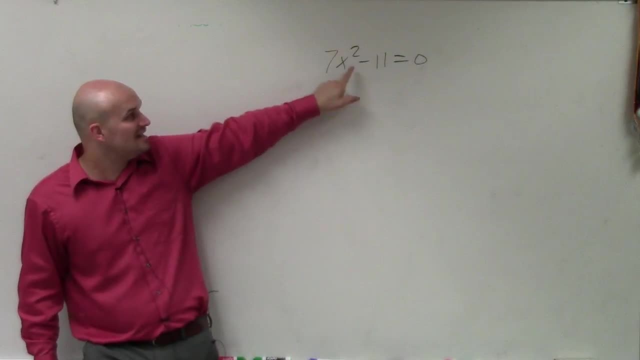 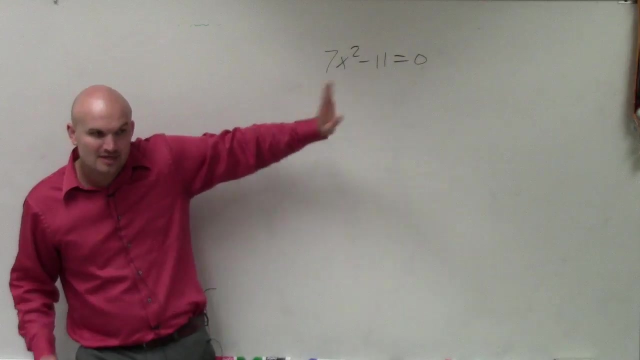 However, in this case, we don't actually have to use factoring because I have my. I only have one variable. When you only have one variable, like a linear equation, we can just use inverse operations. So in this case, this is actually my one example that we're not going to talk about factoring. 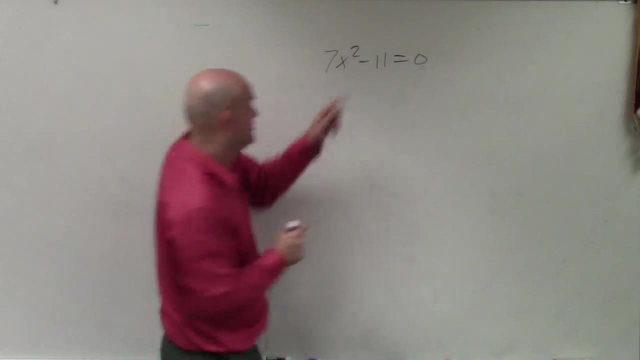 So all I'm going to do is I'm going to undo what's happening to my variable. You can see my variable is being subtracted by 11, excuse me, so I'm going to add 11. Then, so I have 11.. 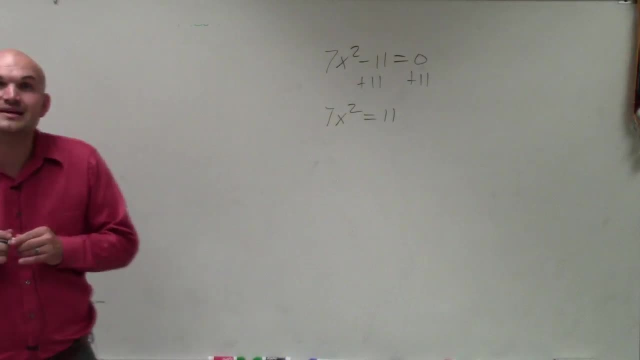 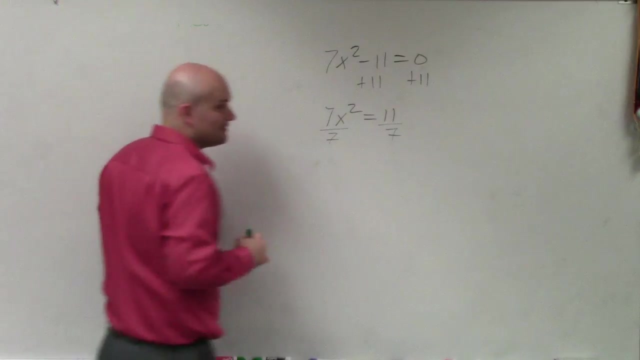 So I have 11.. So I have: 7x squared equals a positive 11. Now my variable x squared is being multiplied by 7. So I'll undo multiplying by 7 by dividing by 7.. Now, 11 does not divide into 7.. 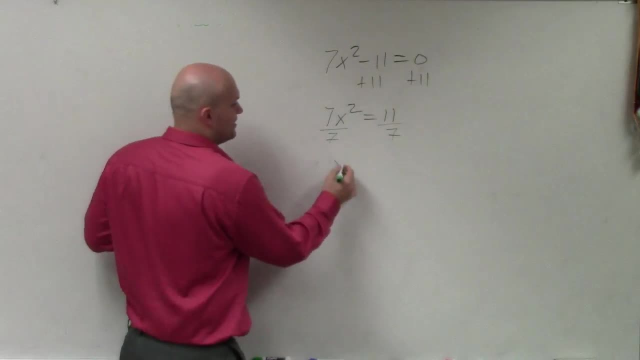 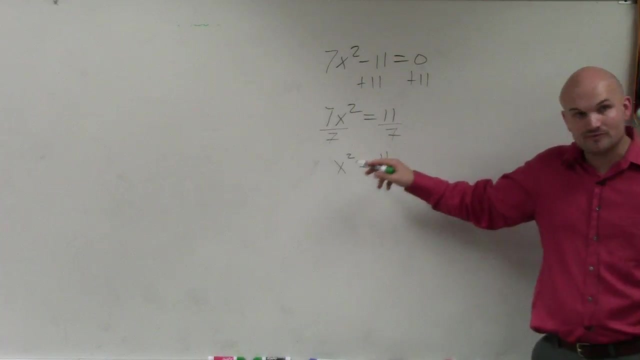 So just leave it as a fraction Fractions are okay. So I have x squared equals 11 over 7.. Now we need to undo the variable being squared. So, using my inverse operations, I can do that by taking the square root. 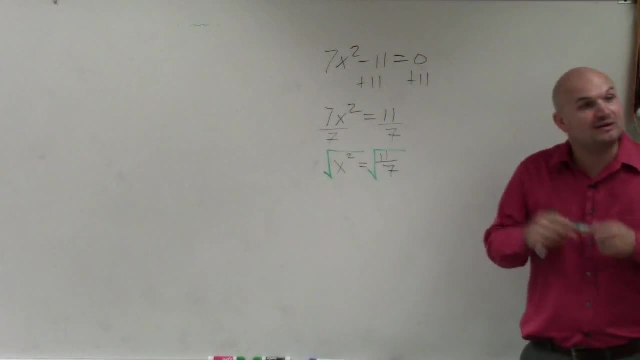 And please remember though, ladies and gentlemen, when you introduce the square root, you have to include the positive and the negative value of the square root. right, The square root, if I had, x squared, equals 4, and I take the square root of both sides. 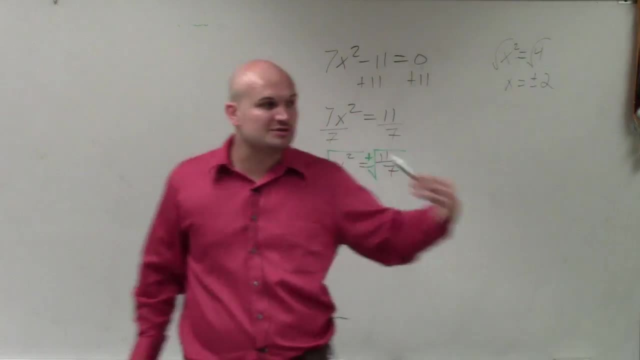 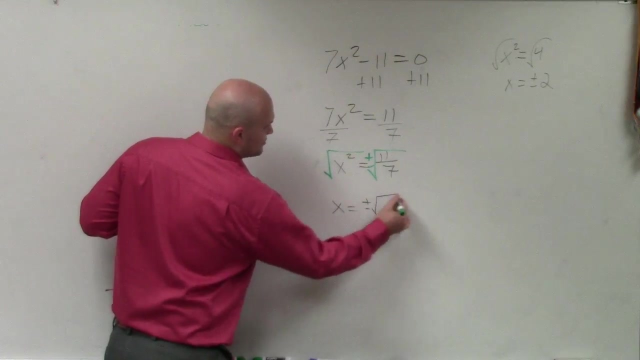 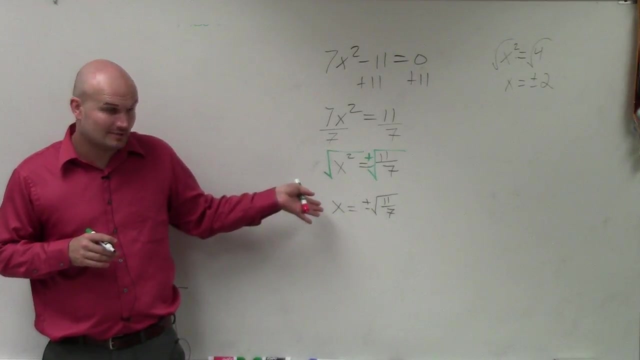 x can equal plus or minus 2, right. So whenever you introduce the square root, make sure you include the positive and the negative. So therefore, x equals plus or minus the square root of 11 over 7.. All right Now, ladies and gentlemen, I don't want to go over your stuff, but from Algebra 2,, 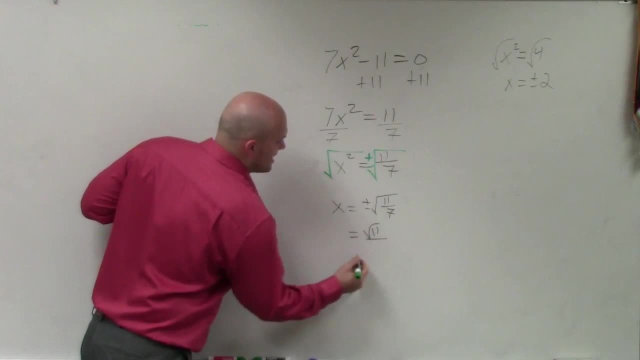 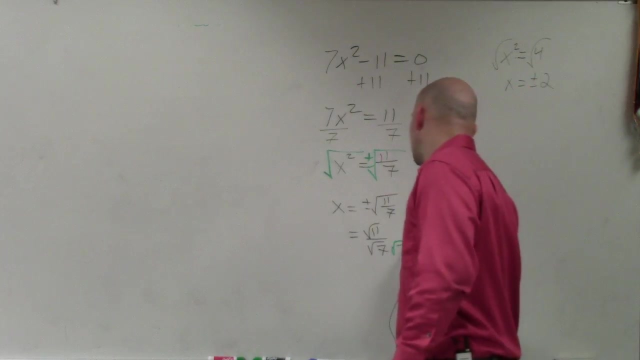 we want to make sure we simplify this to square root of 11 over the square root of 7.. And instead of dividing by the square root of 7, we have to rationalize the denominator. We'll get over this stuff again. We'll go back over this. 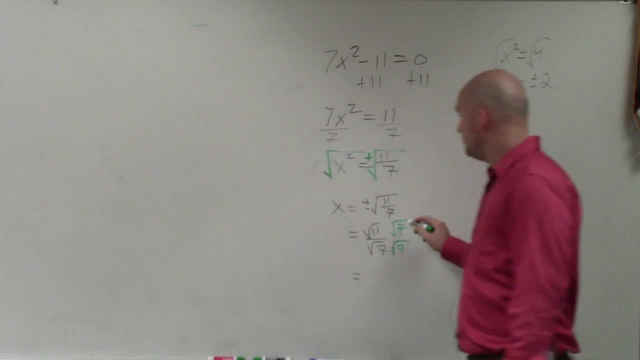 But this is another thing that I just want to remind you of. Then you multiply. square root of 7 times square root of 11 is the square root of 77.. Square root of 7 times square root of 7. Is the square root of 49,, which is just 7.. 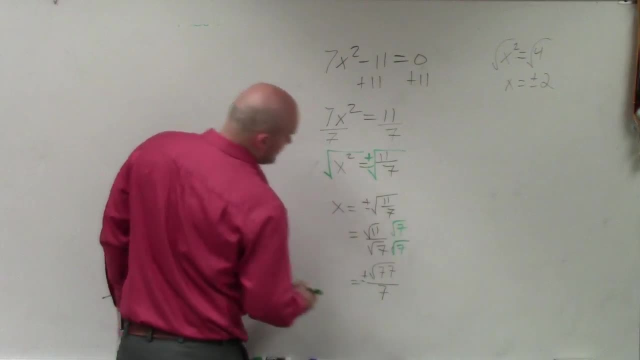 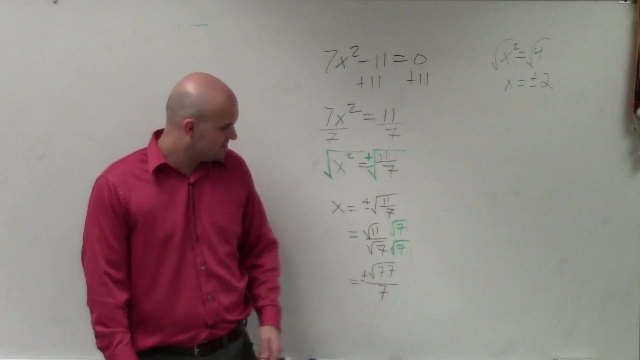 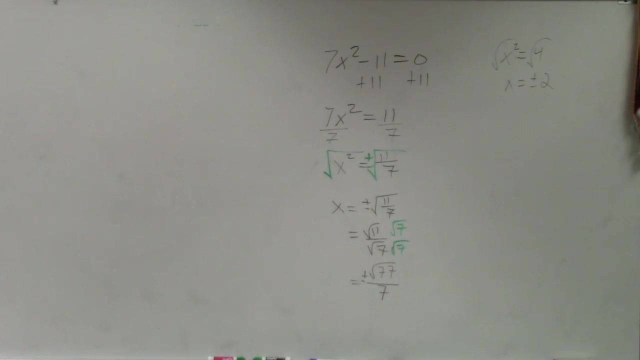 So that would be plus or minus square root of 77 divided by 7, which you cannot divide the 7 into that, because that's the square root of that. But that would be your final answer. Okay, So the first box. all you guys simply need to do is solve for x squared. And once you do that, you're going to get the following: 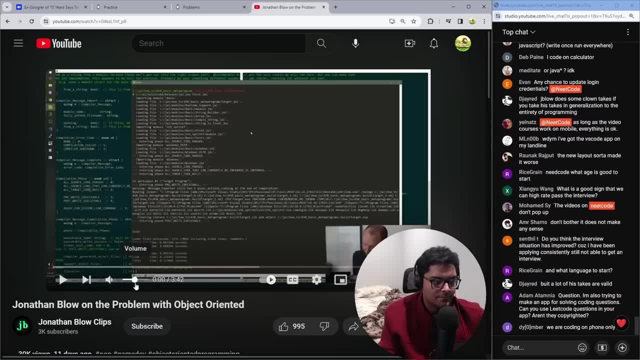 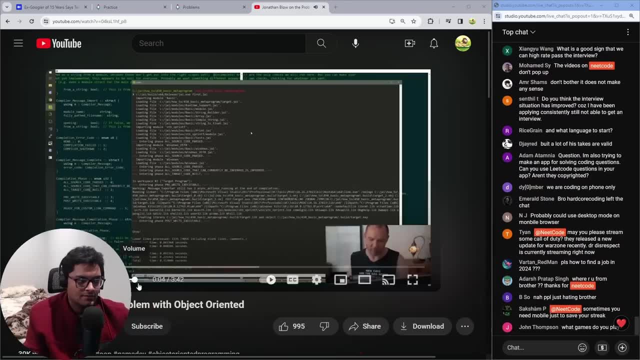 So let's see what he has to say about object-oriented- And I technically pre-watched this, but it's interesting. One of the big problems with software right is that starting in the 80s- prior to the 80s- everybody was just trying to solve real problems and trying to get. 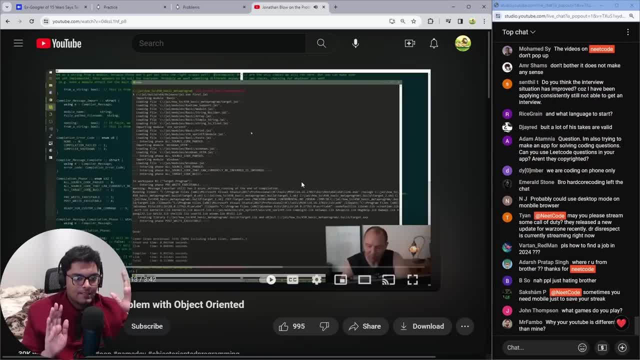 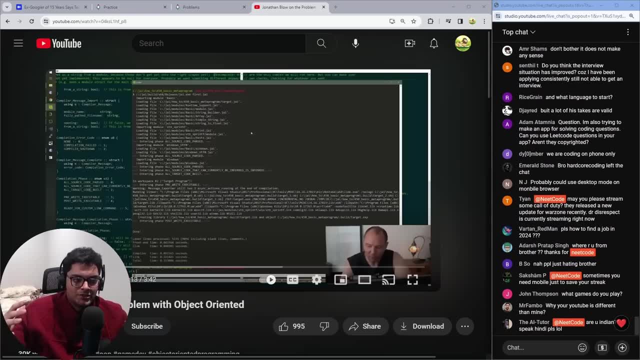 computers to solve real problems, right? I hate to interrupt like 13 seconds into the video, but this is partially what I was saying And I hate too much abstraction. In the older days there was obviously less abstraction because as more time goes on we get better ways of doing. 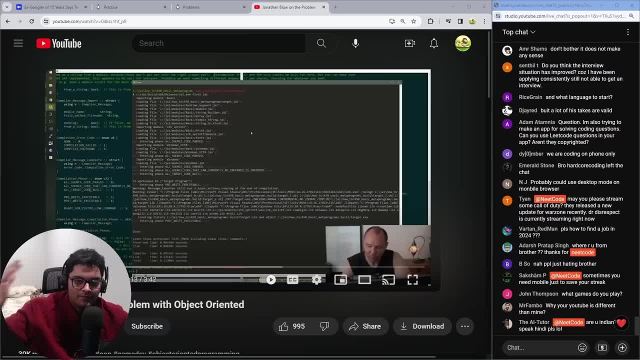 things. higher level programming languages, right Like Java, has more abstraction than something like C, where you are closer to the hardware layer. That's what I mean by the word abstraction, And so this is especially prevalent in front-end development, where you hardly even know what's. 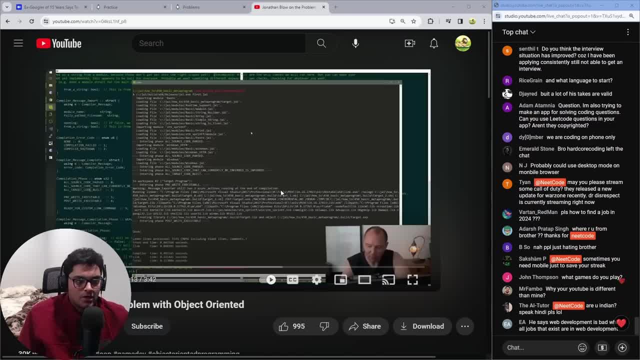 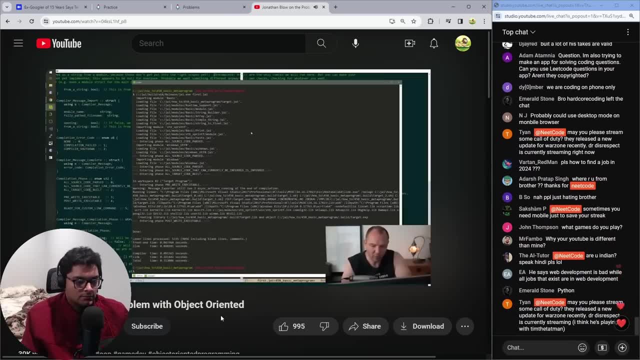 going on under the hood anymore. I bet a lot of front-end developers hardly even know, like what a web API is. But anyways, let's continue. Starting around the 80s, computers got fast enough that you had a lot more leeway around how you solve the problems. 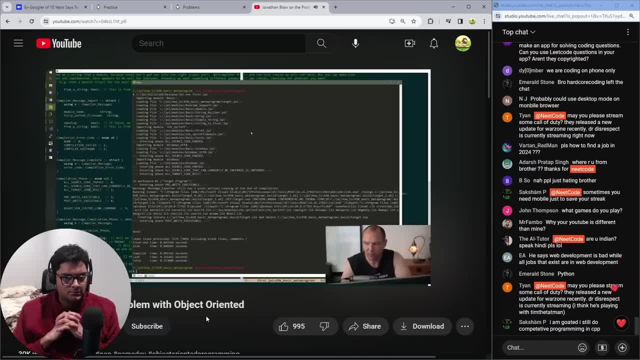 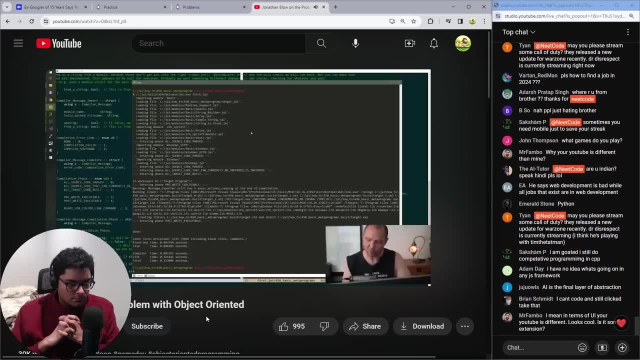 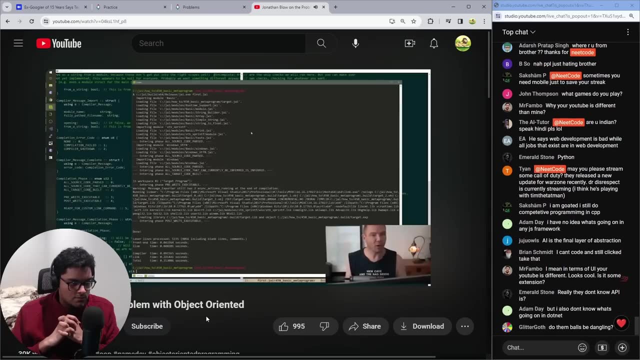 And people started making all these theories about how to solve problems in the best way, And so object-oriented programming is like one of those theories, right? Oh, on the list of things in C++ that are wrong, object-oriented is wrong, right, Because of course, Alan Kay invented the. 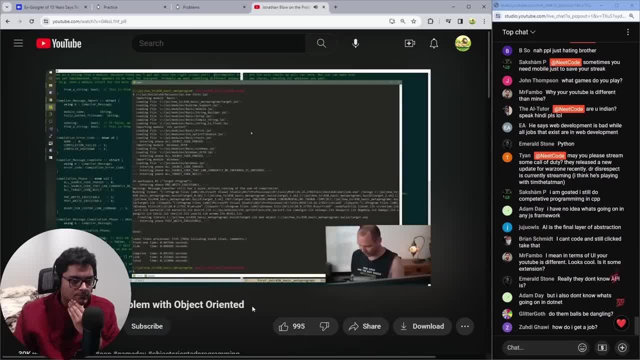 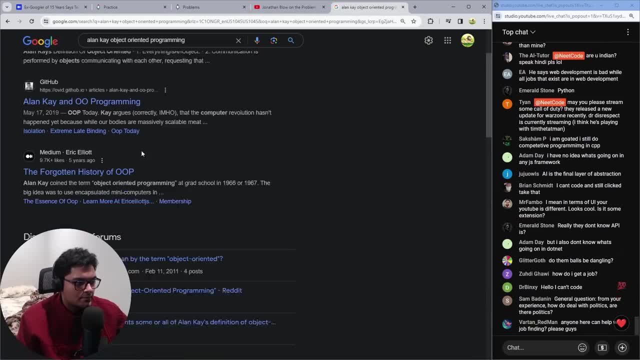 term object-oriented and it meant something else. It meant small talk, not C++. I'm not sure what he's talking about there. I mean, I believe him. I assume he's right. Anybody who's older in programming is usually right. The inventor of the term object-oriented.